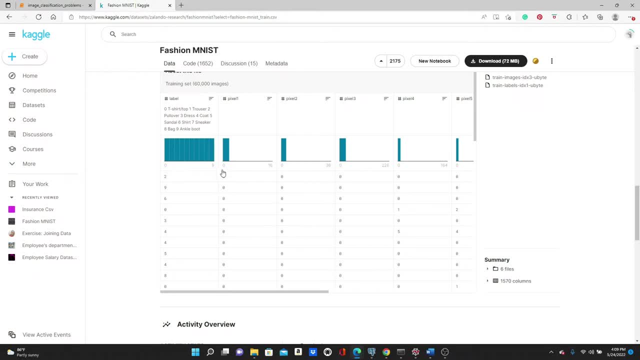 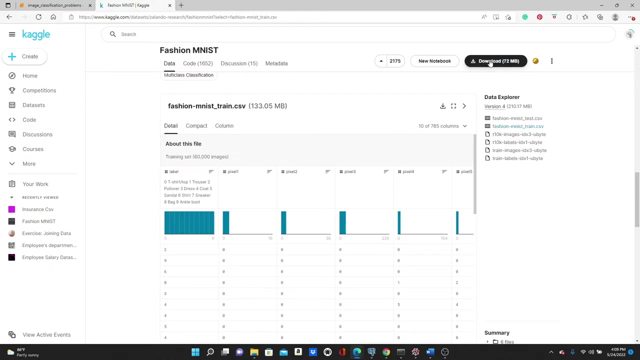 values. but luckily for this data set, we already have the pictures in the pixel form, so I'm going to show you how these pixel forms can form a picture. I have the link of this data set in the description box below. please feel free to click on this download button and download these files and look at it. we 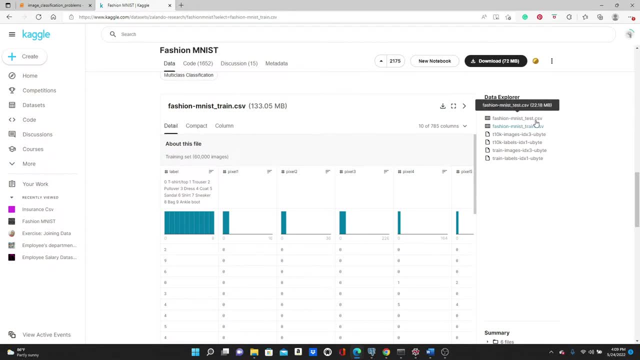 have fashion amnesty train and fashion amnesty test, two separate data set here for training and testing. so we are going to use fashion amnesty train for training the model and fashion amnesty test for testing or evaluating the model. I already downloaded the data set and I already have them saved in the same 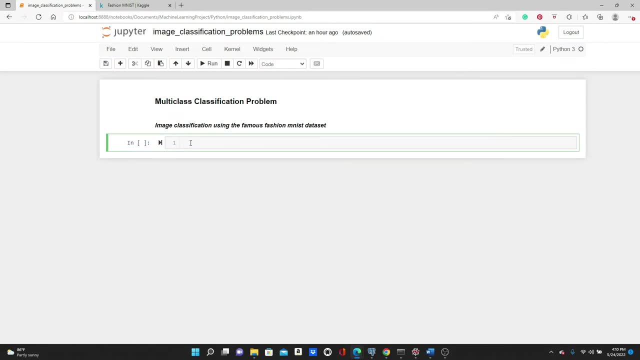 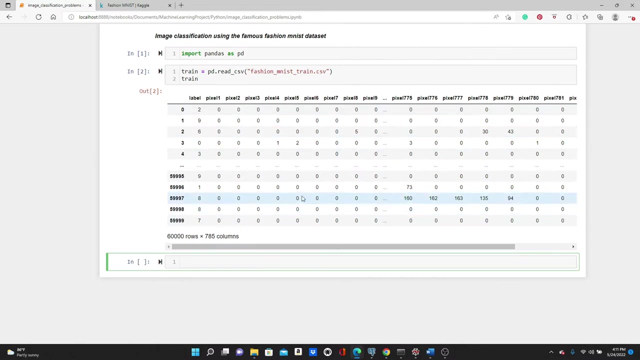 folder as this notebook. so I'm just going to start right now. so import pandas as pd. now let's get the training data set: pd dot. read CSV: fashion amnesty train dot CSV. look at training data set. so we have 60,000 rows of data for training purpose and you can see we have. 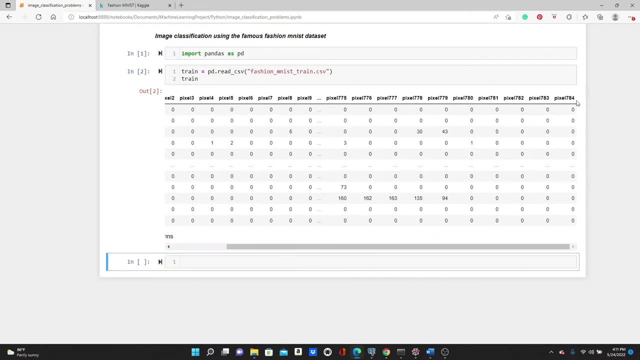 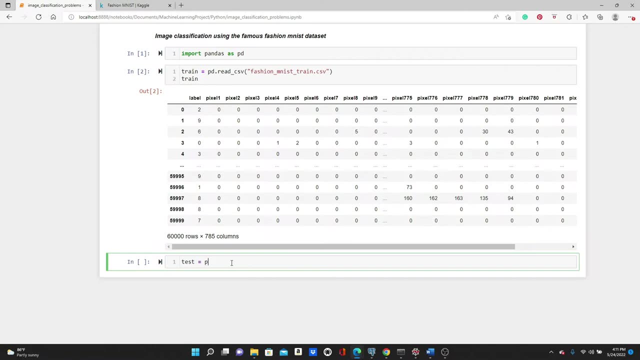 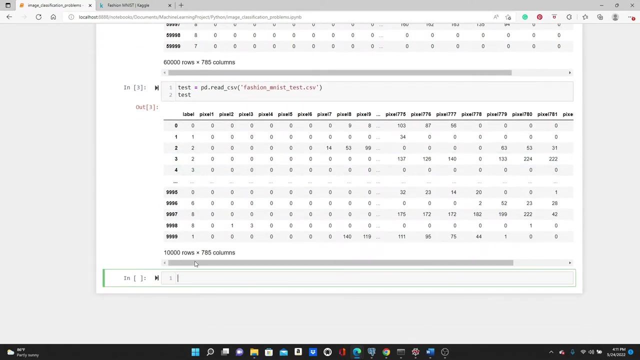 the link to the training data set and we have the training data set and we have the label first and then 784 columns and they are all pixel values. now the test pd dot. read CSV fashion: amnesty test dot. CSV test. here is the test data center. we have 10,000 rows of data as test data set. in last few videos we had to. 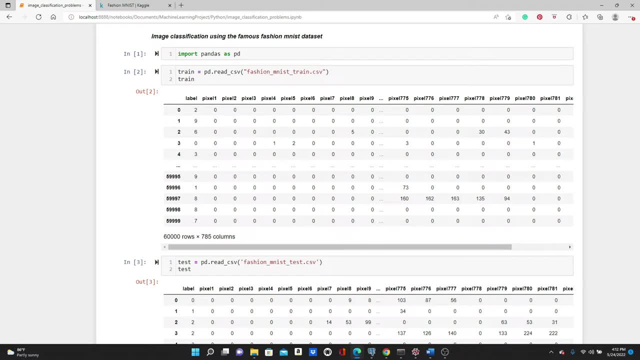 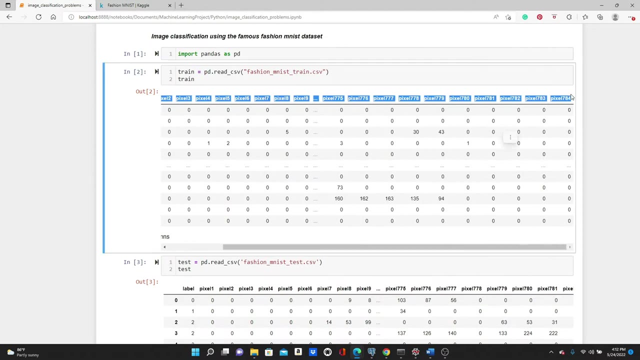 use the train test speed method to split the data set for training and testing. but here we already have it arranged. we have training data set separate and testing separate. we just have to separate the X and wine. so for for training, here X is going to be all the pixels and Y is the label, so it's 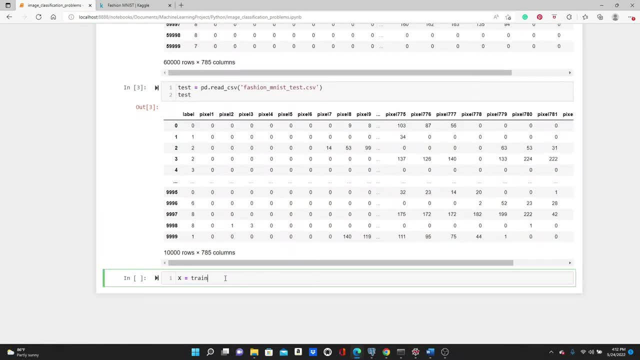 very clear. so X train, dot and drop columns and label all the pixels. so now we have created the entire column and the label is going to be the complete abandoned. now here we have, guys, two columns, the label and, sorry, not eggs. I will use the X train. my train is going to be it train. 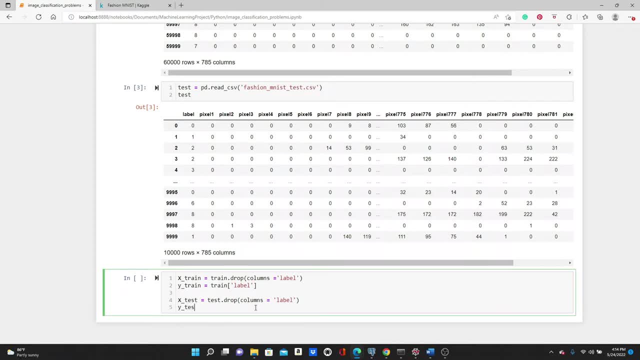 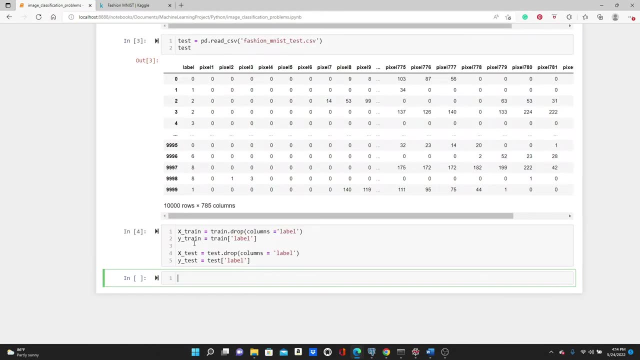 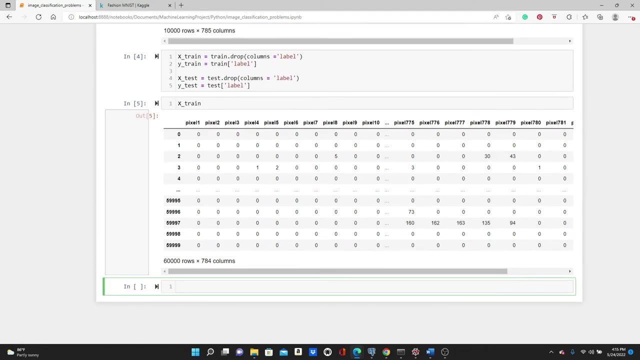 the label X Test is going to be it train label label. so we have x test, x train, y test, y train ready. let's see how x train looks first. here is how x train looks look. we have only the pixel values in the x right now. before diving, 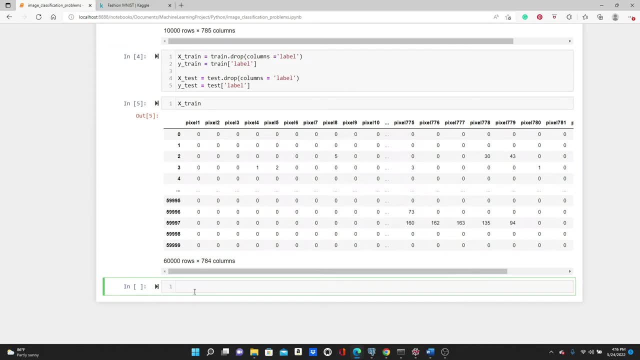 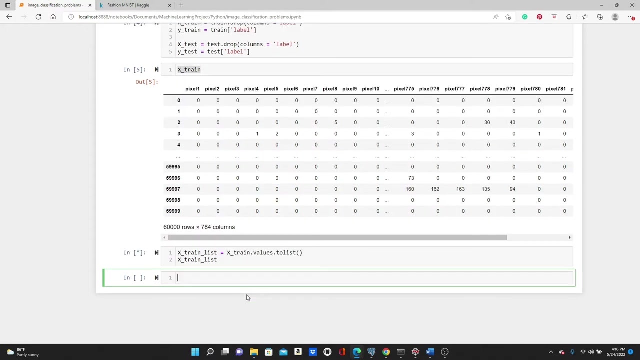 into the model. i want to see some of the pictures, how the pictures actually look like. for convenience, i'm just going to first convert this x train, this data frame, to a list. x train, dot, values, dot to list. so x train list. you can see it is converted to a two-dimensional list. now i'm going to import numpy. 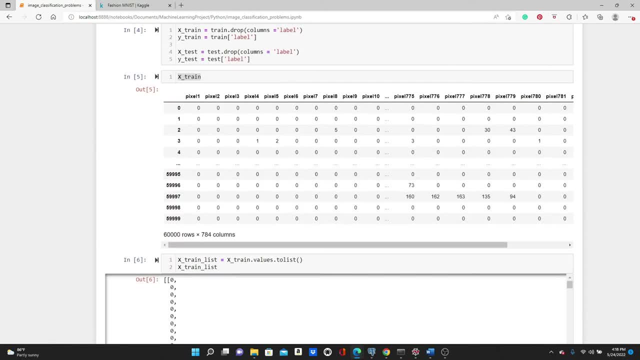 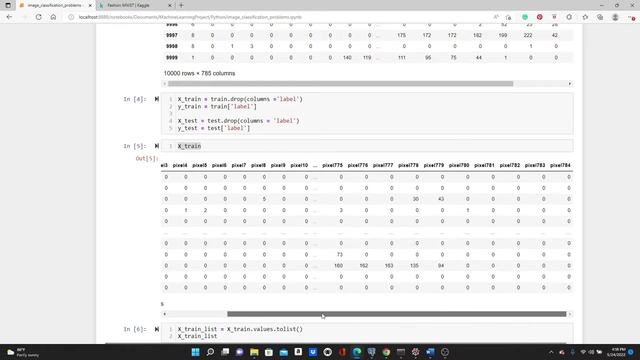 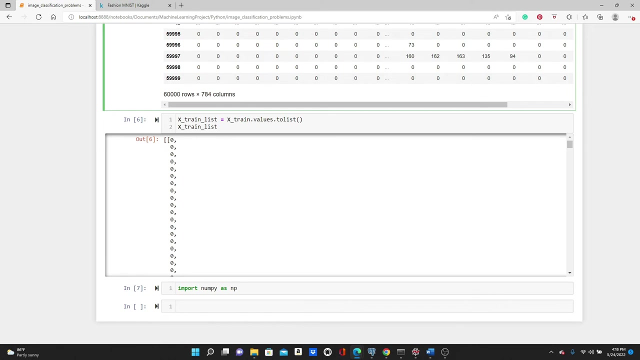 numpy, numpy as np. we will need numpy because, look, each of the images, pixel values are just one dimensional. we're going to reshape them as three-dimensional before we will be able to use and make it the image. so we'll need matplotlib import, matplotlib dot pi, plot s p l t. 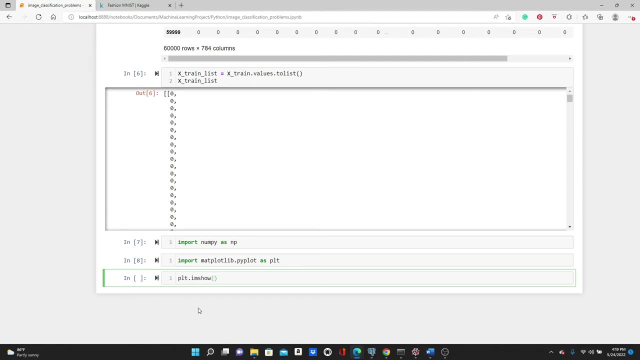 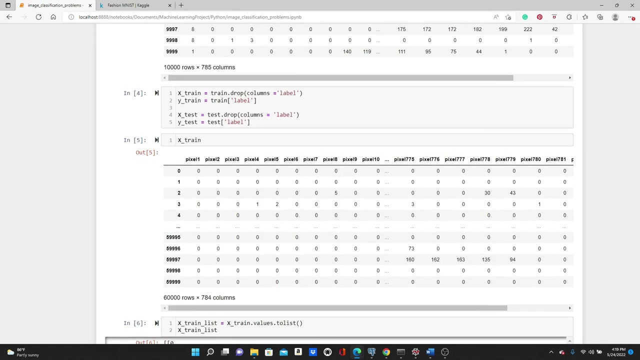 p l t dot. i'm show mp just so buy half sold mp dot. im show mp dot. sorry, mp dot. try to remember here scans mp dot. now- let us look at the whole initiative- comes our first label. we are going to reset our persecution plate and we are going to take our first label. 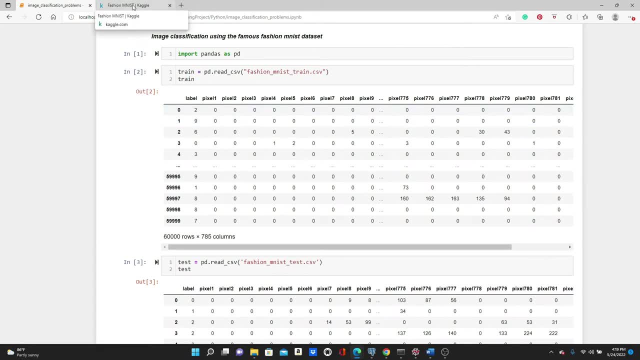 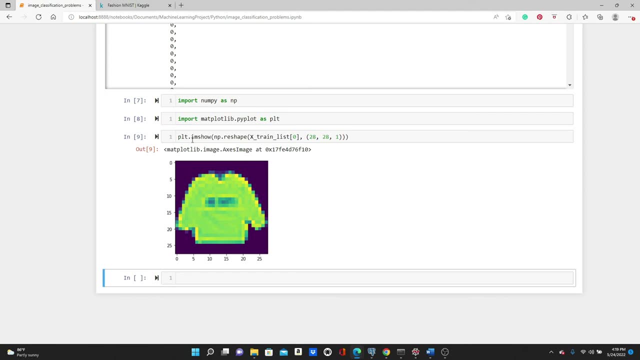 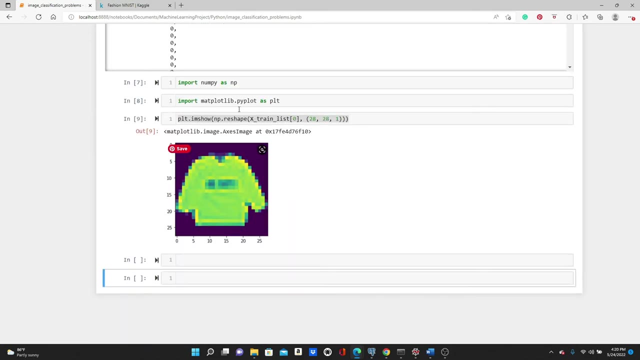 and we are going to use x maintain. so let's see what two is. two is a pullover, so you can see this is a pullover. let's see this one: five, nine, nine, nine, nine. it says that the label is seven. okay, I'll just copy and paste. 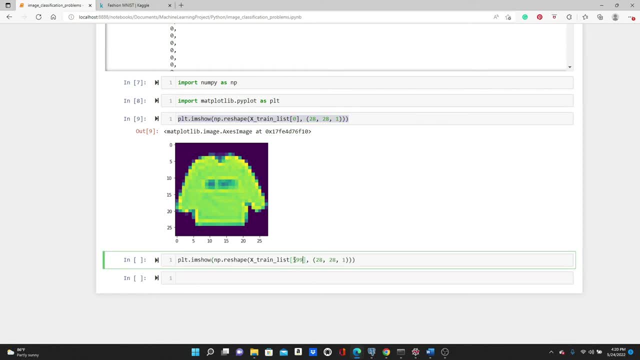 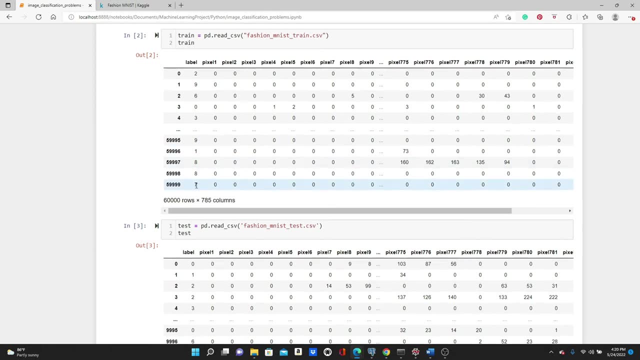 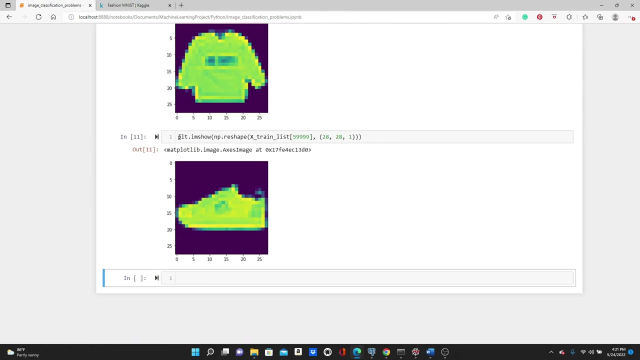 five, nine, nine, nine, nine. okay, it says label seven, right, label seven. label seven was a sneaker, so we saw it's a sneakers picture. let's see some more. 12, it's an echo boot. then a what about 20? 20 looks like a handbag. so you see some of the pictures, how they look like. 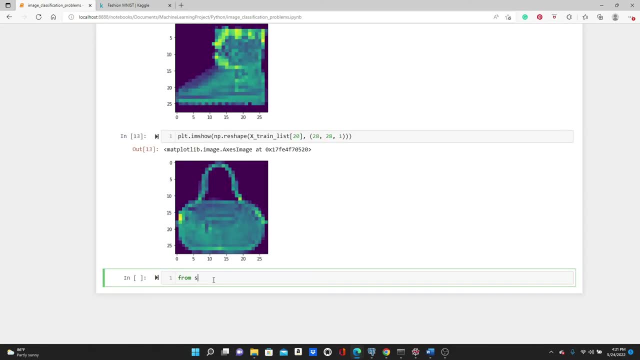 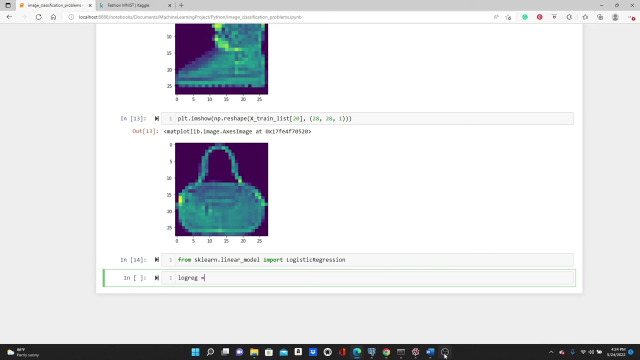 let's dive into the logistic regression problem. first, from sk learn dot linear model: import logistic regression. next step is going to be just save an instance of logistic regression model and also train the data set in the same line. logistic regression, random state: uh, 12. fit extreme Y train. model training is done. and remember, model training may take a little bit. 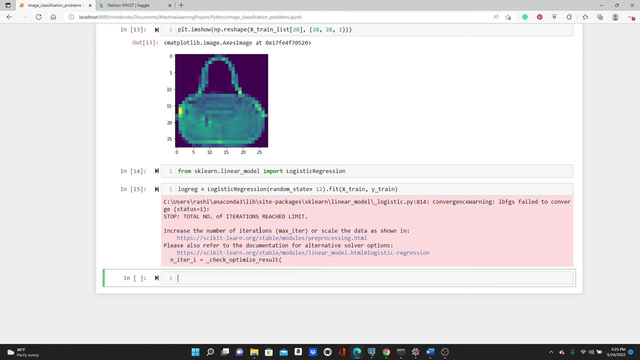 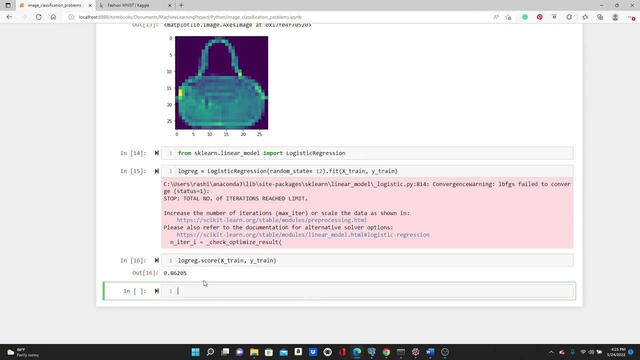 of time because we have 60 000 rows of data and we have a little bit of warning here, but we can ignore it. let's see what is the accuracy of the model. logreg, the score extreme wine cream. it's 86 percent. look, 86 percent of the time this model can detect any of these images correctly. 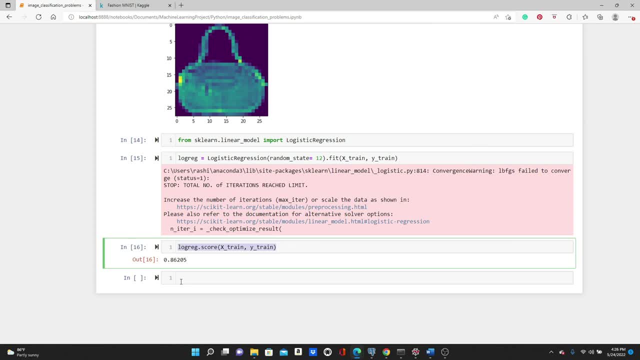 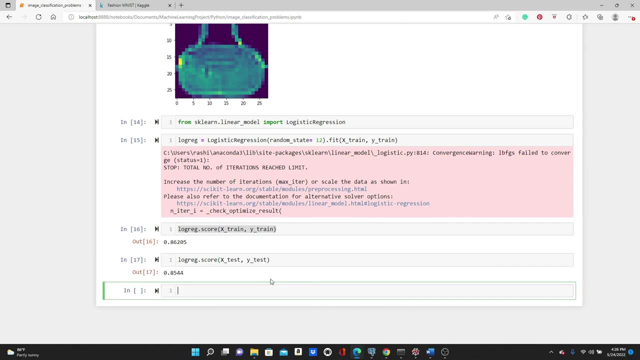 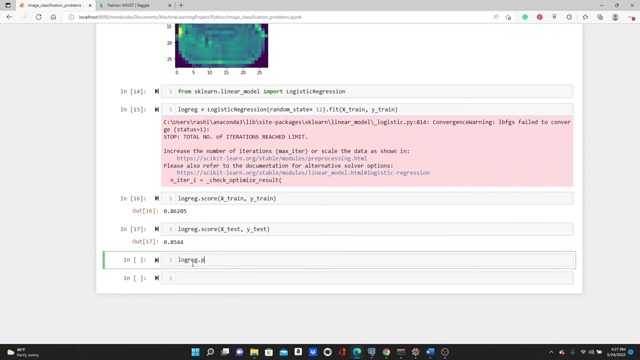 but let's check actually how well it works on the test set. why test 85 percent? pretty good, good, okay, let's check the model another way: dot credit, uh x. queen list. i'll give 5. okay, you have to put them in another bracket. it says zero. so let's check.